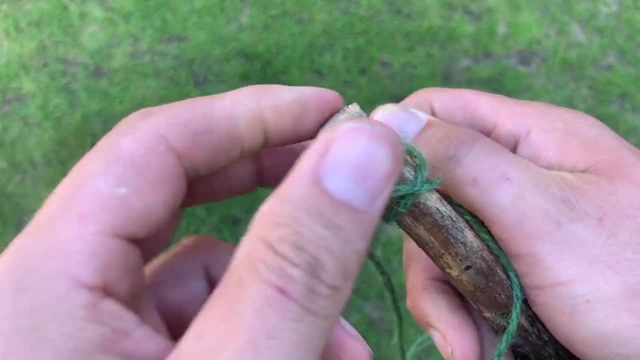 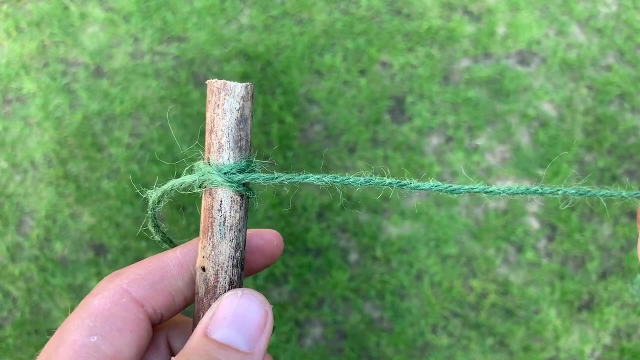 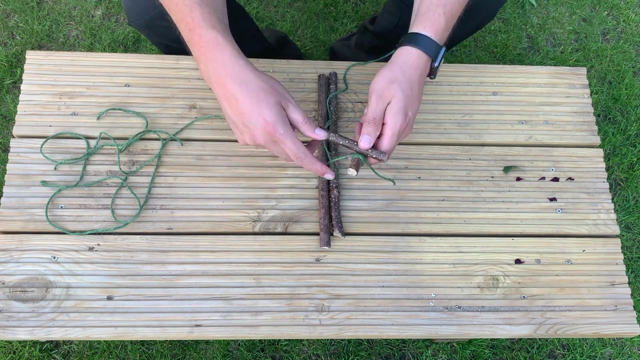 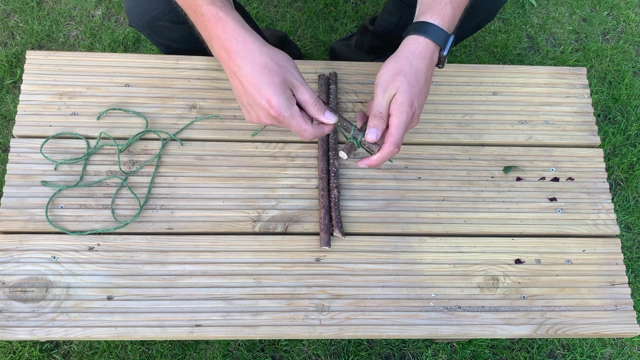 pull tight and that gives us our clove hitch. Then have your second stick opposite. we're going to go over that one under that one, over and under. We keep doing that a couple of times to make our square lashing Over under, over under. and then you can cinch round, pull it really tight and tie it off. 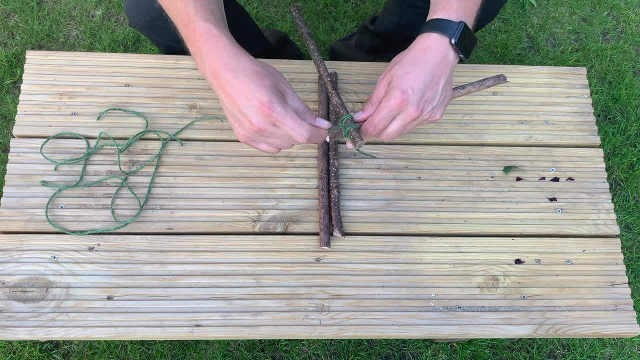 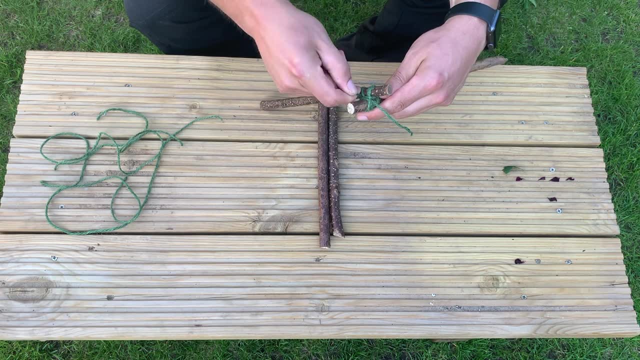 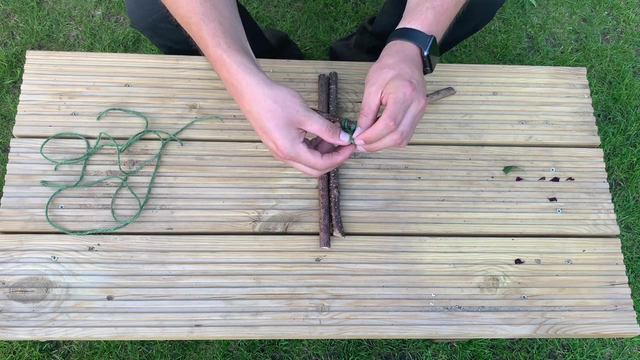 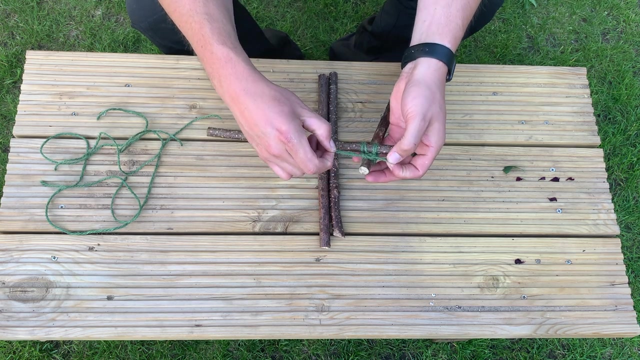 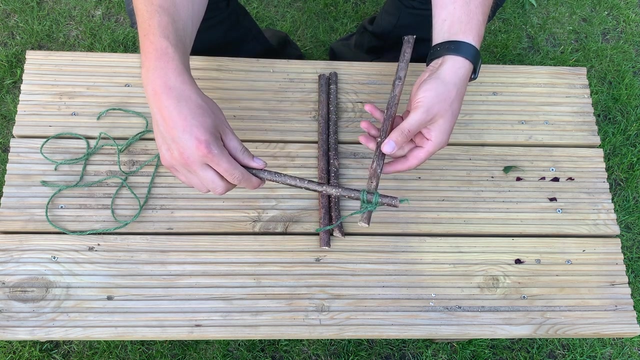 And you can pull it up and over under, and then over and over and over, and then you can cinch around, pull it really tight and tie it off, and tie it off. so that's one corner done and I'm just going to make the others 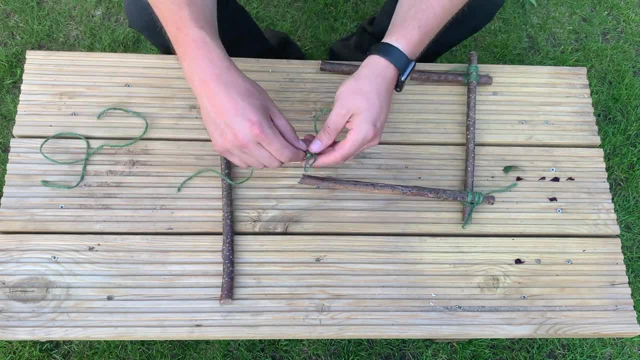 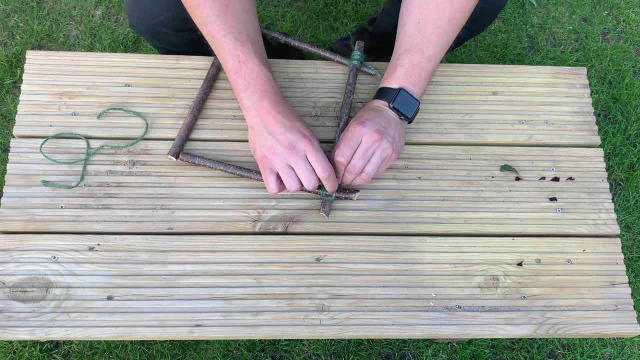 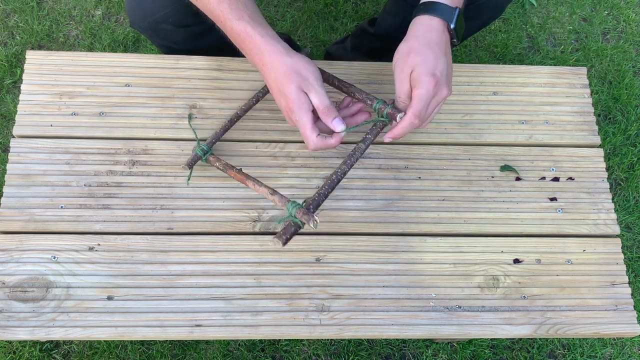 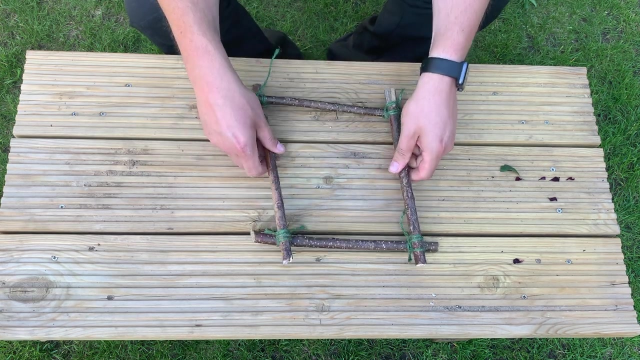 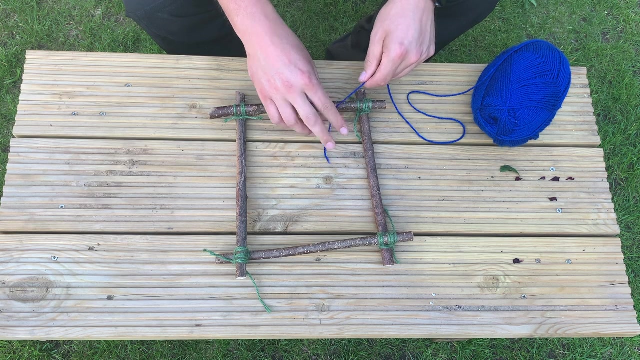 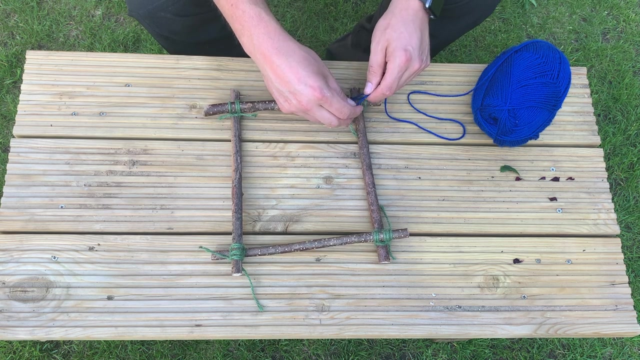 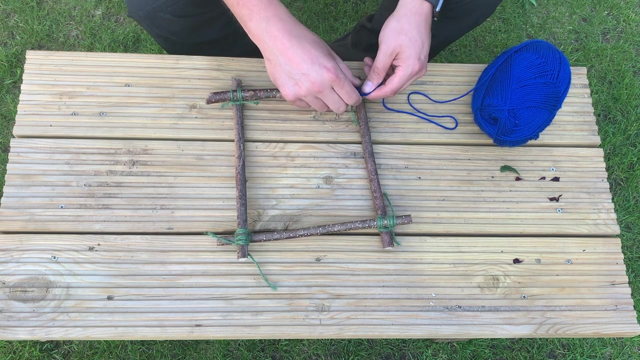 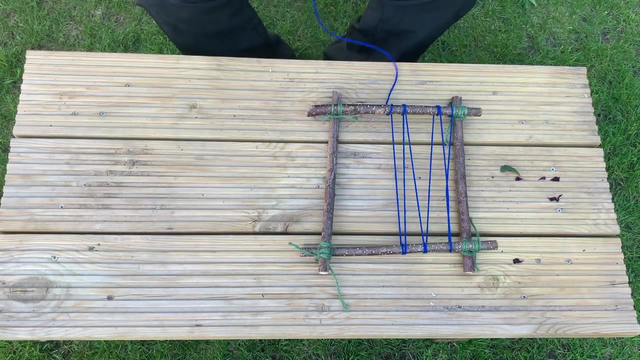 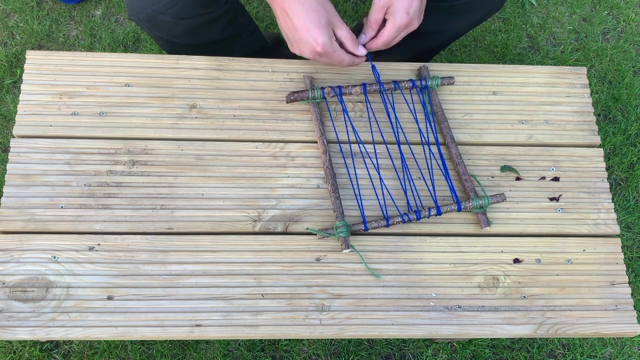 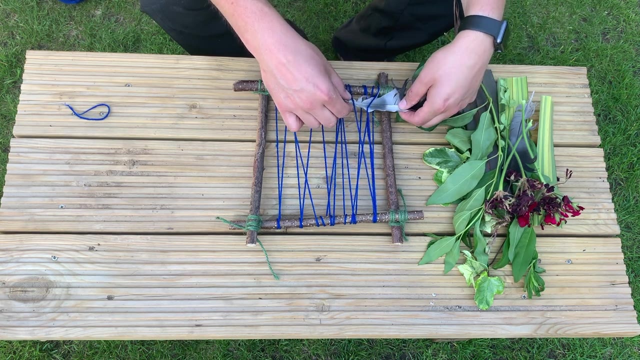 as I wouldn't frame. the next job is to tie on a piece of wool or thread that you have. we're going to use this to cross the frame so that we can weave in between them. then the thing to do is to find some natural items in your garden or